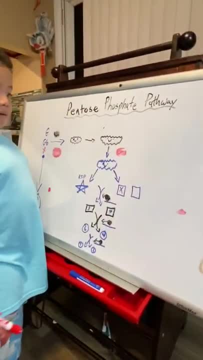 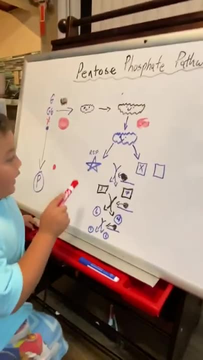 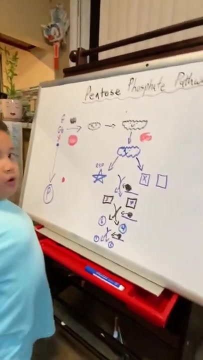 ribose 5-phosphate. If it epimerizes, it becomes xylose 5-phosphate. Now if ribose 5-phosphate and xylose 5-phosphate join, they make these two molecules. You might hear one of them from: 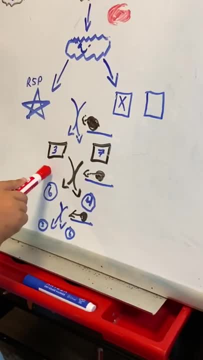 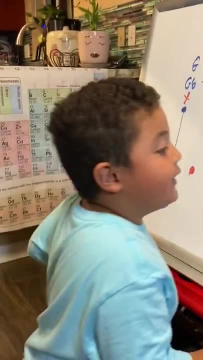 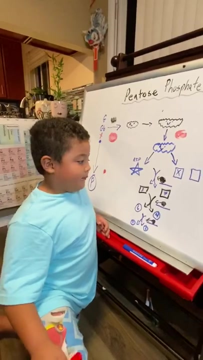 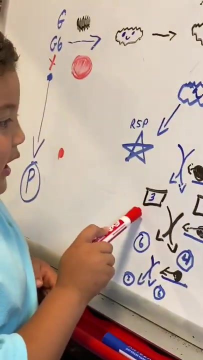 the glycosis pathway. Here's glycerol high 3-phosphate from the glycosis pathway and central heptose 7-phosphate- Kids say that word a couple times. How A transketoase enzyme. Now central heptose 7-phosphate and glycerol high 3-phosphate. those two molecules are 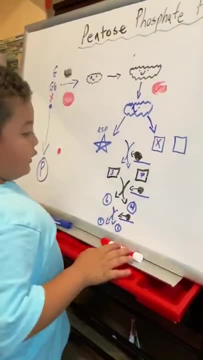 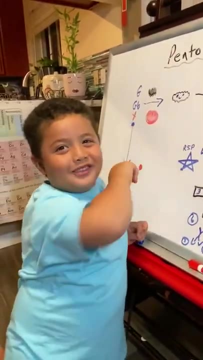 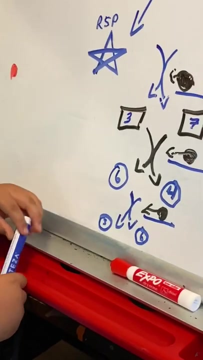 going to join again To make what You might hear. you might hear one of. you might hear why we couldn't go to fructose 6-phosphate. Kids Becomes becomes A rethoraceous 4-phosphate and fructose 6-phosphate. How Transandoly Vous rider en gaye. 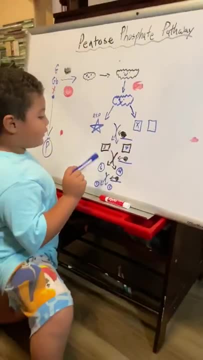 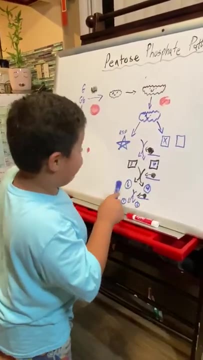 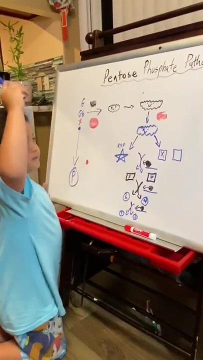 Kids Now guess why we couldn't go here? Because guess where fructose 6-phosphate was Right here the whole time. Fructose 6-phosphate leaves and goes to the glycolic pathway. oh no, and here comes xylose 5-phosphate. and now said and now, 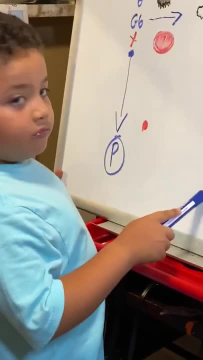 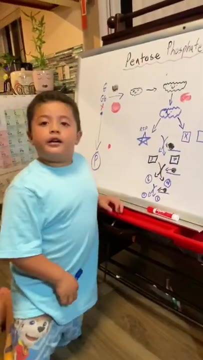 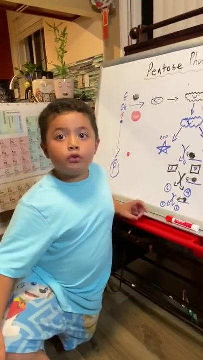 erythro is 4-phosphate and xylose 5-phosphate join, they make the last two molecules bursaride hide 3-phosphate and ribob bursaride hide 3-phosphate and fructose 6-phosphate. 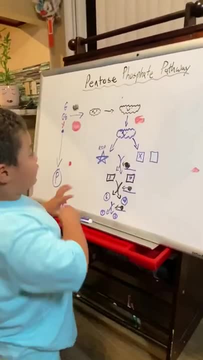 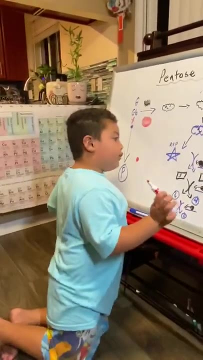 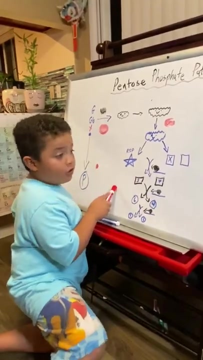 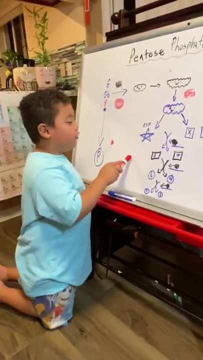 kids. and do you know? there's a, there's a line here, kids, you wonder what this is. you wonder what the line for the oxidative phase and the non-oxidative phase. the oxidative phase is breaking down, the non-oxidative phase is slopping molecules. kids.